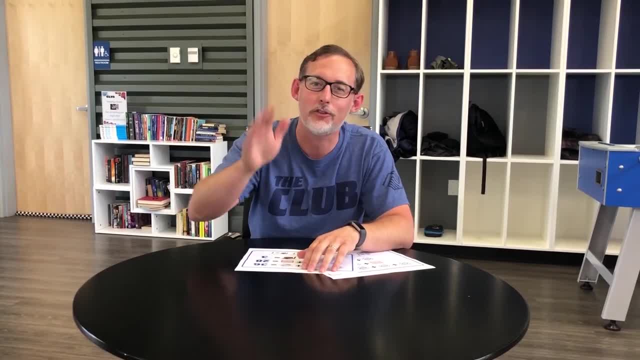 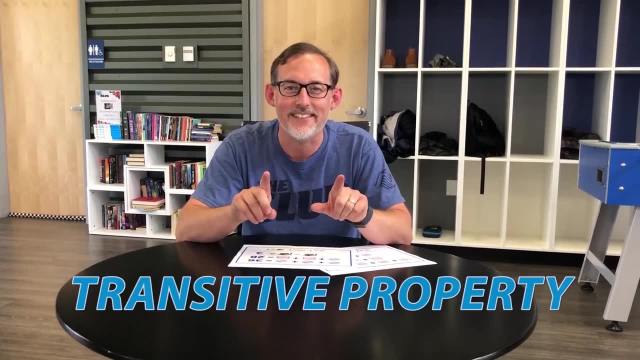 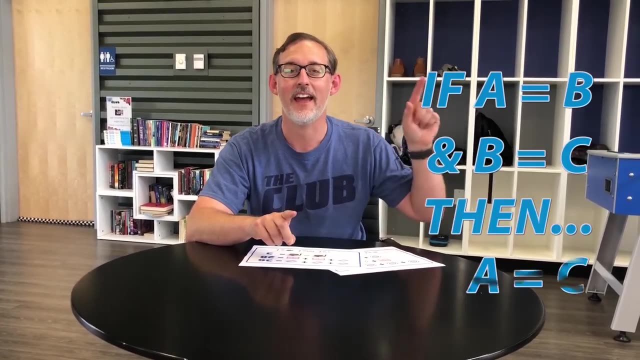 connection. So one example that you'll find out in high school- and I know most of you are younger than high school, but as a really cool principle you can Google- it called the transitive property, And what that means is this: If A equals B and B equals C, then A equals C. If, then, That's logic. 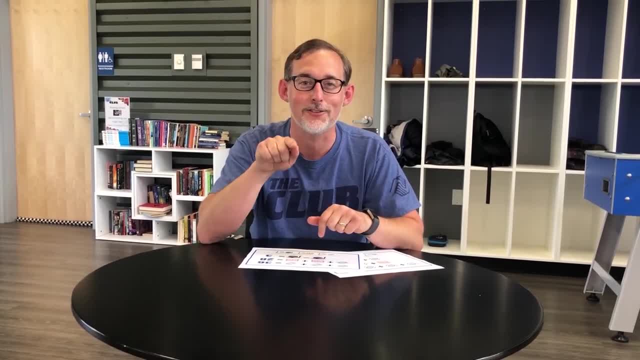 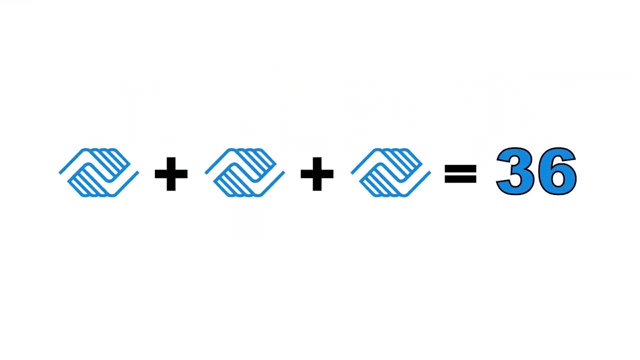 So today we're going to do logic puzzles And put your brains to the test. Let me show you one. So we're going to start with a pretty straightforward one. So let's start with the hands, this top row. What we've got is hands plus. 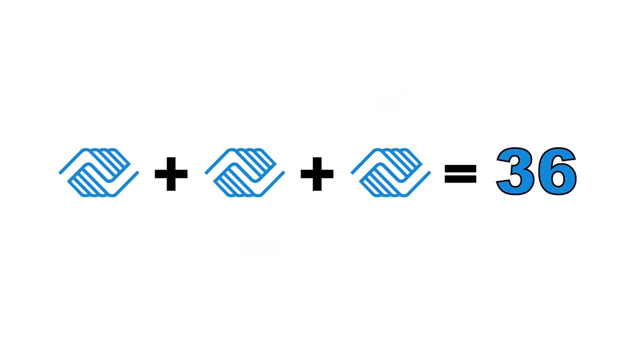 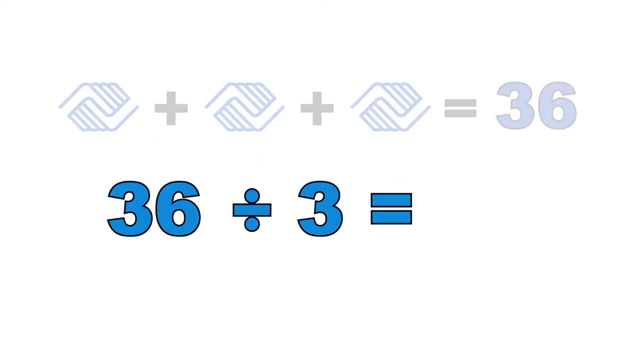 hands plus hands equals 36.. If the hands are the same and we know what they are, then all we have to do is take 36 and divide it by three, And so you might need some help doing this. But if we know that these three numbers are the same, what three numbers that are the same when added together? 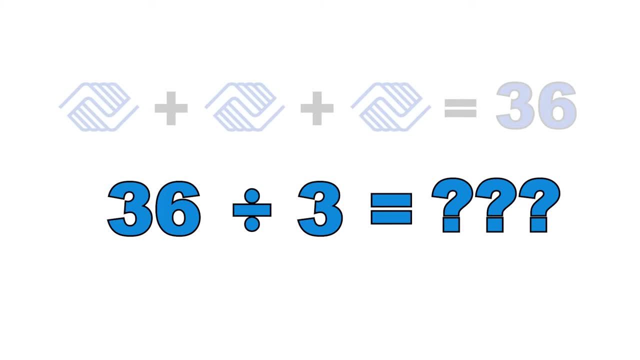 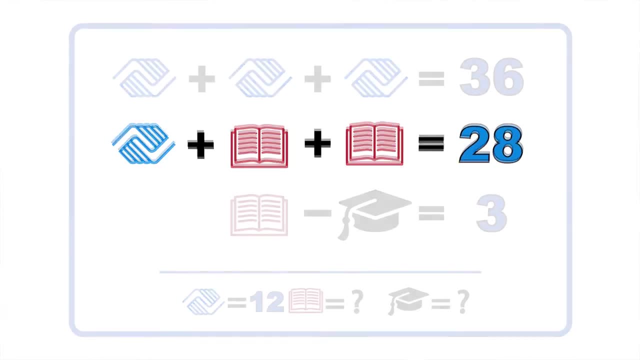 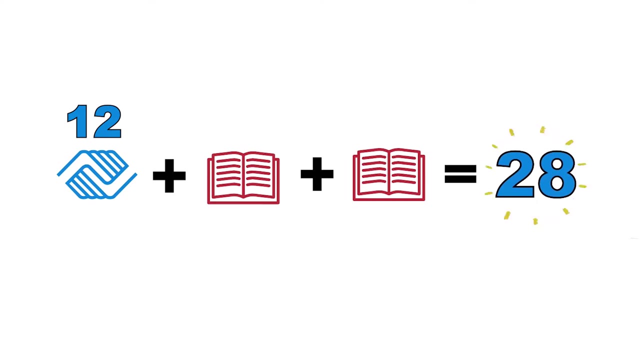 equal 36? And a quick division problem. Well, I'm going to tell you that the answer is 12.. So hands equals 12.. That allows us to go to the next one. So now we know that those hands are 12.. So 12 plus a book plus a book equals 28.. How do we figure that out? 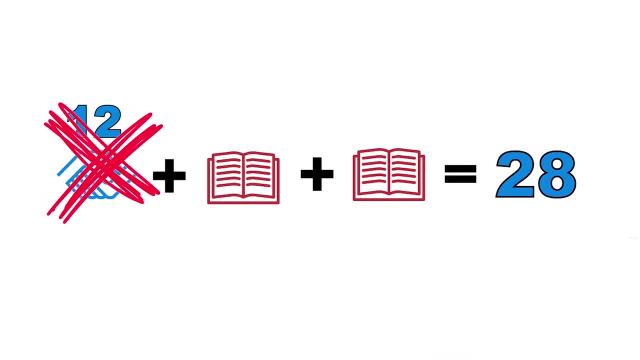 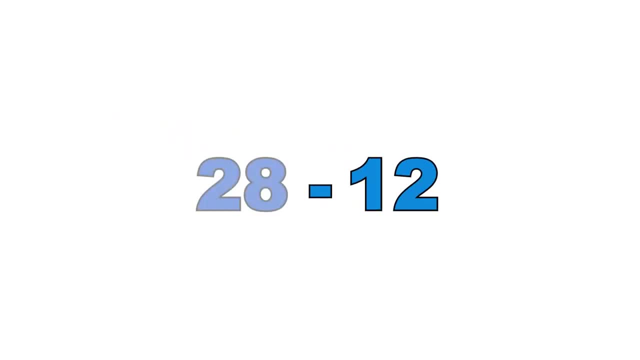 So the first thing you want to do is you got to get rid of the hands, just like an algebra problem which you learn about in middle school. So what we're going to do is we're going to actually take the hands 12 and subtract that from 28.. 28 minus 12.. 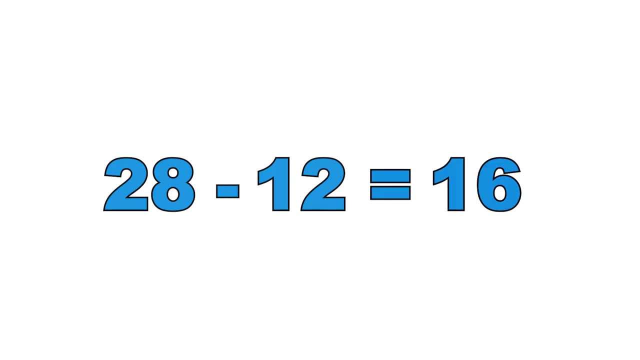 equals 16.. So if the book is the same, which we know, it is: what plus what equals 16. if it's the same number, Is it 4 plus 4? No, that equals 8.. Or 6 plus 6? No, that equals 12.. 8 plus 8? That? 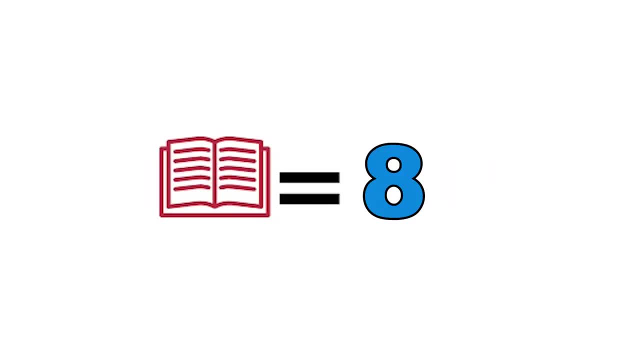 equals 16.. So we know that the book is 8.. So we are almost there, now that we know that the book is 8.. So if the book is 8, this last equation is maybe one of the easiest ones to figure out. 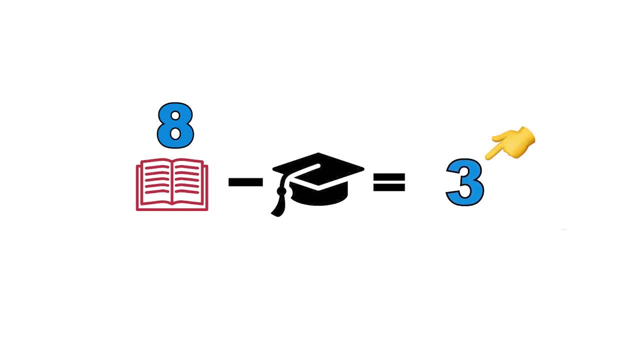 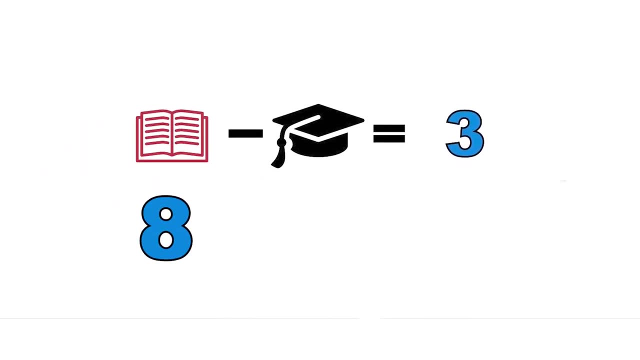 because 8 minus what equals 3? What is that cap? What number is it? And if you think about it for a while and do some work on it, you'll realize that 8 minus 5 equals 3.. So the cap equals 5..